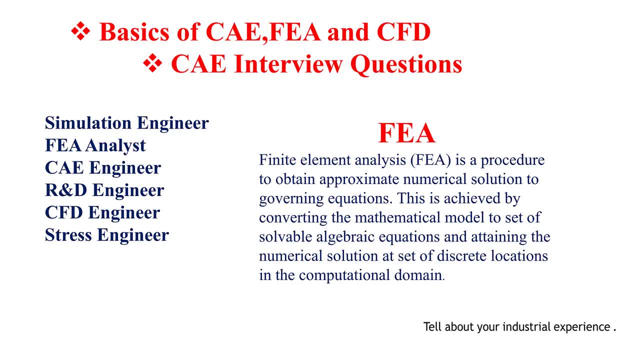 questions. Okay, so add your industrial experience in a well-defined manner and execute it in a better manner. Okay, the plus point When it comes to this FEA. so what exactly it is the term FEA? Okay, so what exactly it is the term FEA? Okay, so what exactly it is the term FEA? 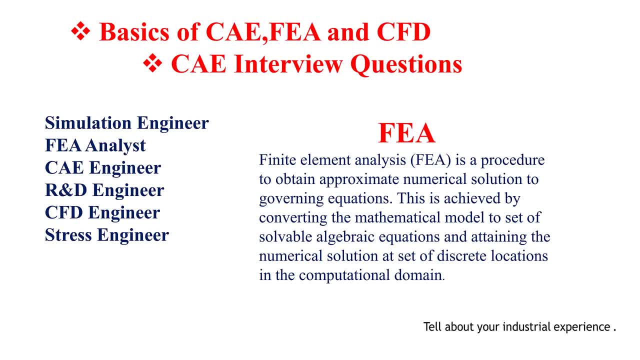 So, in short, finite element analysis is the method to solve the numerical equations dealing with the entire model consisting that one. So we're going to just discretize this. discretize it in the form of small elements, Okay, and once you convert that particular entire model, 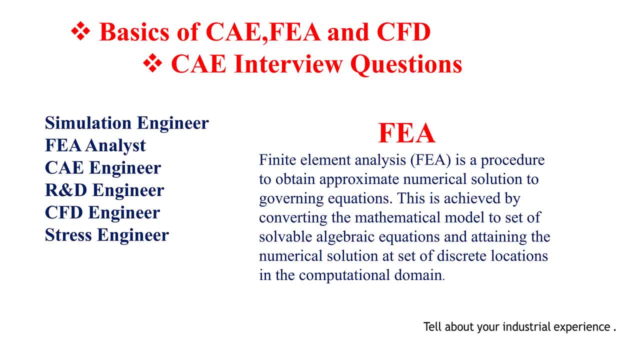 into simple mesh. we are going to apply the boundary conditions and solve for the results. okay, so this is what exactly we're going to do there. so, when it comes to technical terms, so it's a process where exactly we're going to just deal with the approximate numerical solution to the governing equations. okay, to achieve this, 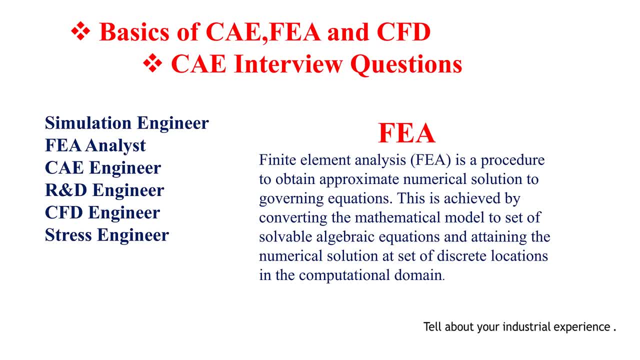 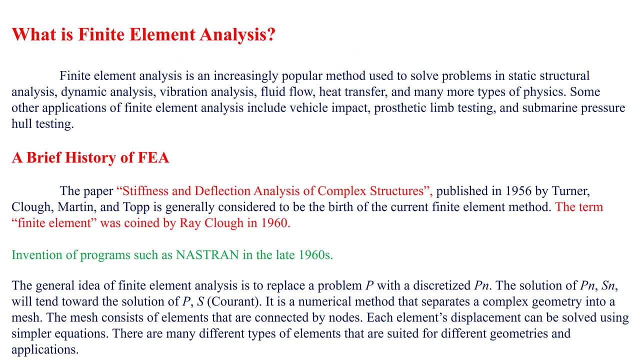 what exactly we're going to do is. so we're going to convert these mathematical model to a set of algebraic equations and we'll solve them to get the results. okay, in short and simple, we can say yeah. so here the same question again. so this particular method, that is, finite element analysis, 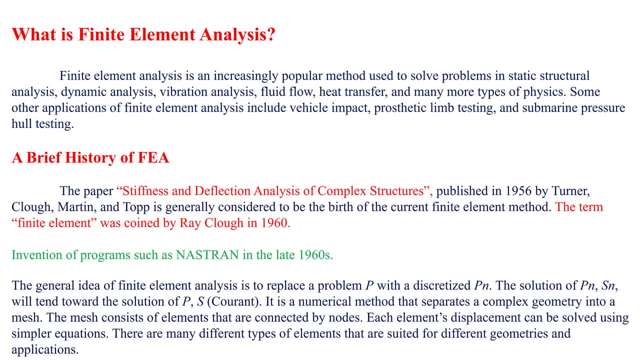 is popularly used to deal with the structure analysis, the dynamic analysis, vibration, heat transfer, fluid flow c of t and all and and many for physics okay, even like the vehicle impact and the drop test analysis, even the pressure vessel analysis, even we can consider this submarine pressure hull testing and all. 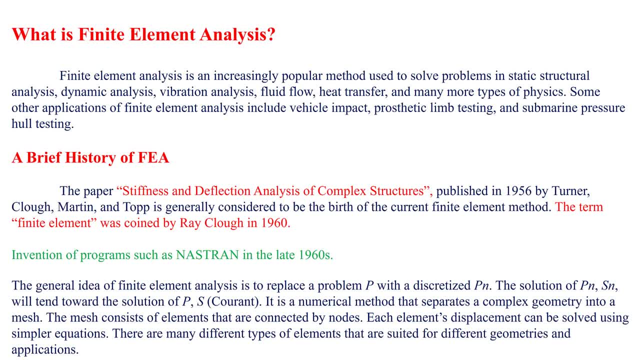 so in these all the domains we're going to use this finite element analysis. so when it comes to history of this fea, so the paper that is, stiffness and deflection analysis of complex structures, which is published in 1956 by t turner and clough martin and toff, is generally considered to be the birth of finite element method. 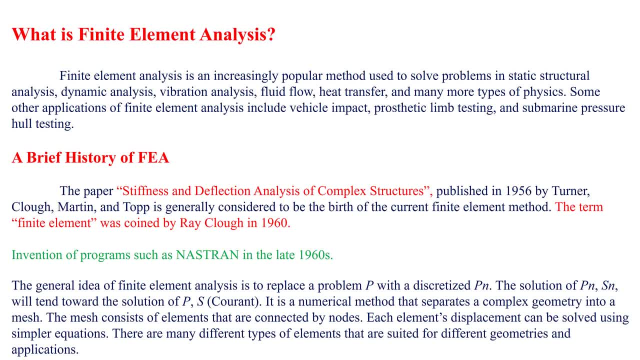 okay, during 1956, so in the year 1960, the finite element term was coined by ray clough. even during the same year, the program invented- that is an ex-nastan, sorry, it was just nastan, okay. and meanwhile all the programs like the answers and amicus and so on. well, so generally this finite element. 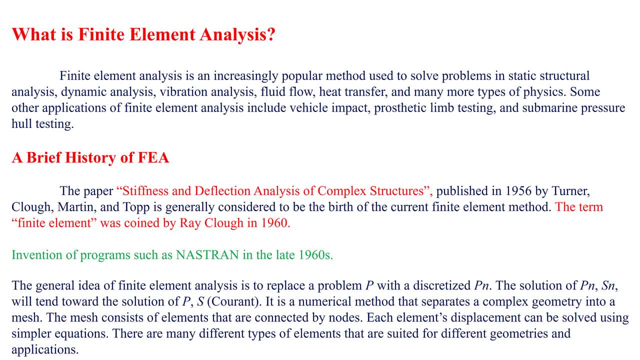 analysis is to replace the problem P, we can consider, with a discretization, that is P, n, if you consider, and the solution of this particular P, n and SN will tend towards the solution of the P and S. okay, so it's a numerical method which will just separate the complex geometry into a mesh. okay, so, as I told, 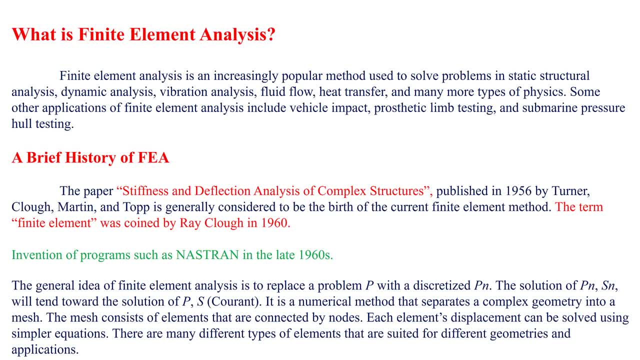 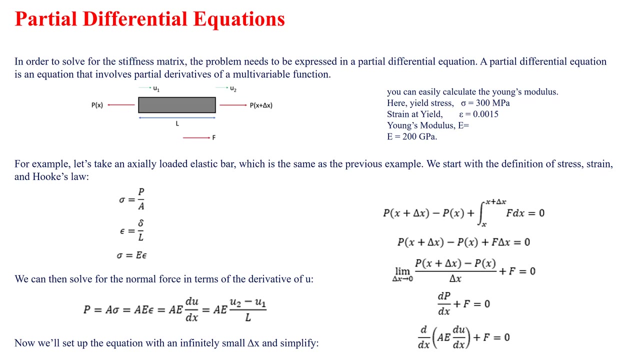 discretization. this mesh consists of elements that are connected by nodes, so so each elements displacement can be solved using this particular equations, the partisan partial differential equations and others, and finally, you gonna get the results. yep, we will see about this. partial differential equations and equation of 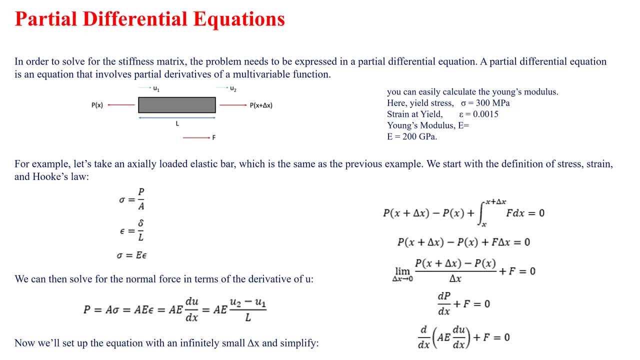 motions now. so to solve this stiffness matrix, okay, the problem needs to be expressed in the form of the partial differential equation. so we already know that. so if you are new to the basics of CAE, remember the partial differential equations will be used to solve these all the numerical models. okay. so this: 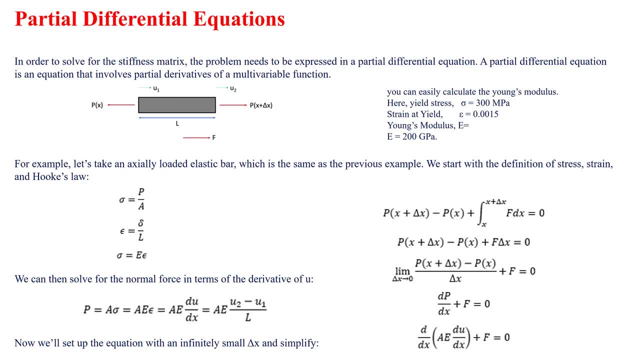 particular equation is called the partial differential equation and it is based on the partial derivative of the multivariable functions. so if you consider the basics, okay, so let's say if I consider the simple bar with the axial loading condition, okay, so which will just follow the Hooke's law in under the 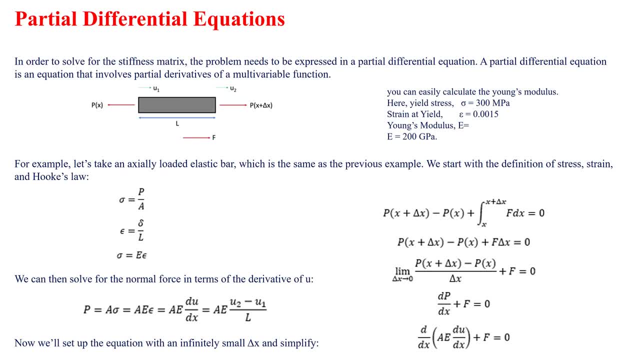 elastic limit. okay, so if you want to just take that one into a normal analysis method, we can start with the definition of the stress strain and the Hooke's law. so once you construct this stress, the formula is the load divided by cross-sectional area. right, the strain, we define it as change. 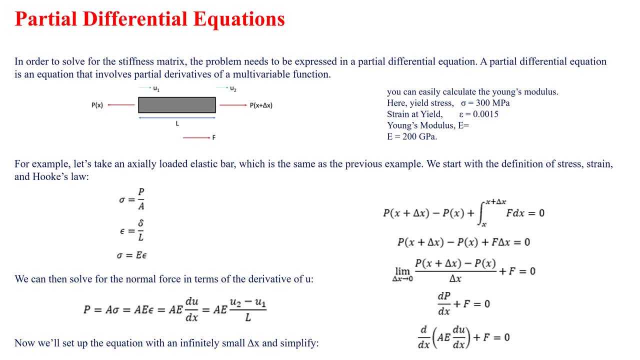 in length to the length like the original length. okay, so when it comes to Hooke's law, it is Hengst modulus which is equal to stress by strain. so where stress which is equal to Hengst modulus has been 2. And stress by strain is equal to stress by strain, equal to stress by strain, which is equal to stress. 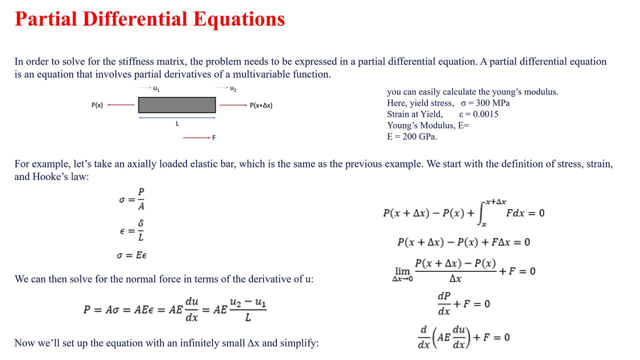 stress, which is equal to x modulus into strain. so again this equation can be just again reconstructed. you could see the load, which is equal to area into stress and that we can just add up the stress value. it is ae by strain, e is the x modulus. so once you again add into the 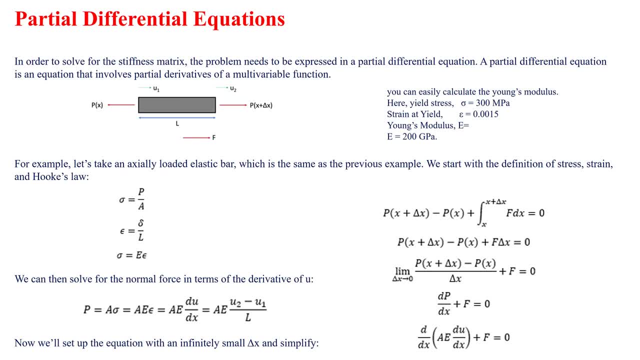 derivatives. it is ae into du by dx, so it is change in length to the original length, u2 minus u1 divided by l. we can consider if you consider the above particular scenario into account. so once you solve for delta x, the final derivative is d by dx of ae into change in length to the 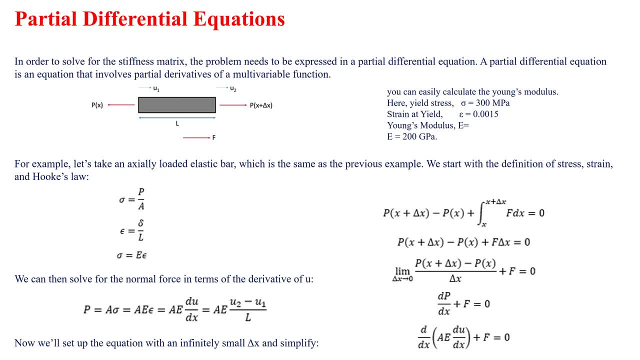 original length plus force, which is equal to 0. so this is how we gonna form the equations. so now, what exactly inks? modulus is so very important term. so you could see there i have given an example for you. if you take steel, or example like the material properties, like yield stress, which is equal to 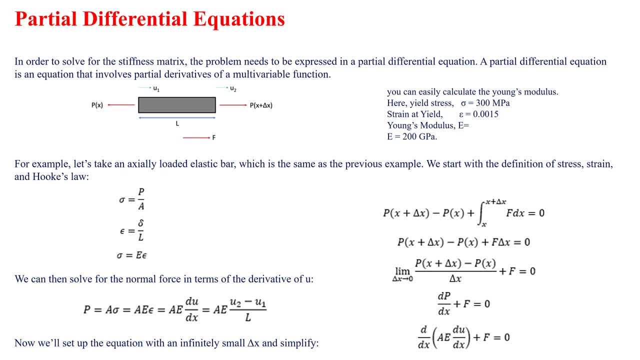 300 megapascal. when it comes to strain, the value is given. so inks modulus is stress by strain, so it is 15 into 2 is 30, so it is the value here, that is, 200 gigapascal, or 20, 10 to 5 pascal. okay, one newton. 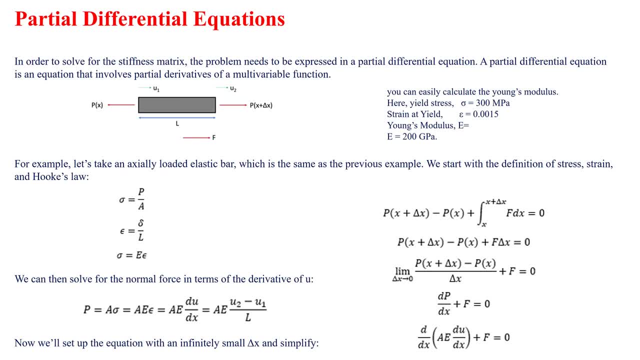 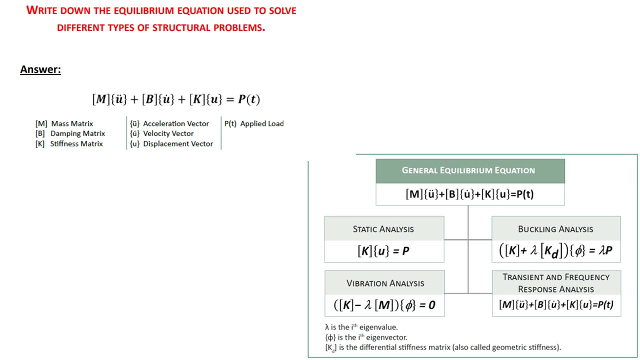 a meter square, which is equal to one pascal. okay, remember that. so this is how we're going to just formulate these things. i hope it's clear. this is quite simple. yep, so here, when it comes to the uh equilibrium equation, the formula you could see here is the: 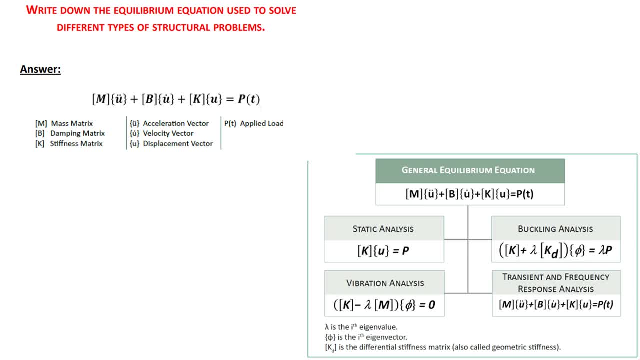 general equilibrium equation, which is equal to uh. stiffness matrix into distance, which is equal to uh. that is f of t. that is the static analysis formula. when it comes to the overall equilibrium equation, that is m, is the mass matrix into acceleration, plus damping matrix into velocity, plus stiffness matrix into displacement, which is equal to. 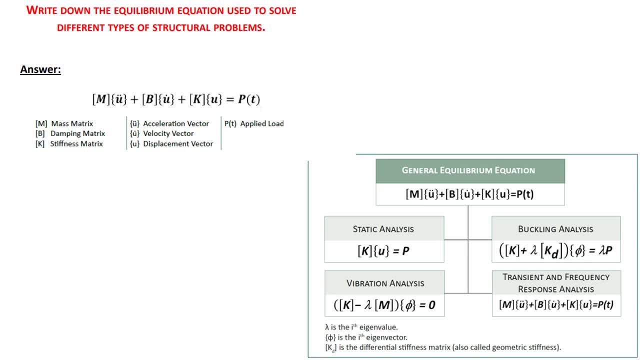 this is p of t that is applied load. so just uh, at the right side corner you could see. for the static analysis, as i said, it is stiffness matrix, that is uh, displacement, which is equal to p, run wood for buckling. the formula is: the vibration is same thing. when it comes to the time based and 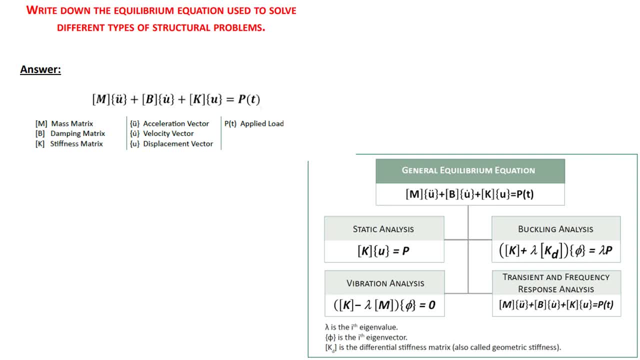 frequency based dynamic analysis. the formula is the final one. okay, so this equation you need to remember so they might ask you during the interviews. the uh terms of basics also you should remember this formula. okay, for the static analysis, this uh mass and the damping will just be a constant, or we can consider it as zero. it will be converted into static analysis. okay, fine. 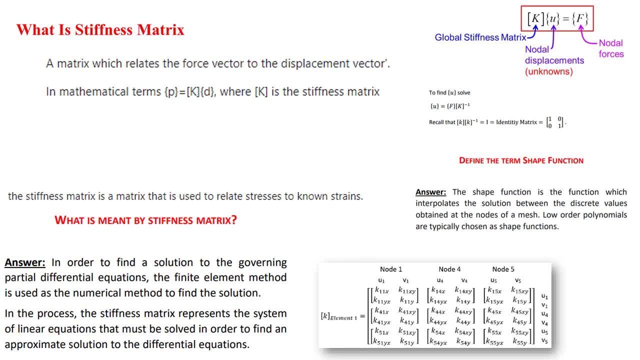 to elaborate more about this stiffness matrix. in short, if i consider f is equal to k, into u, that is, global stiffness matrix- into displacement, which is equal to nodal force. this, simply, the stiffness matrix is used to relate the stress to known strengths. okay, uh, you could see the explanation below. so, in order to find the solution for the uh partial, 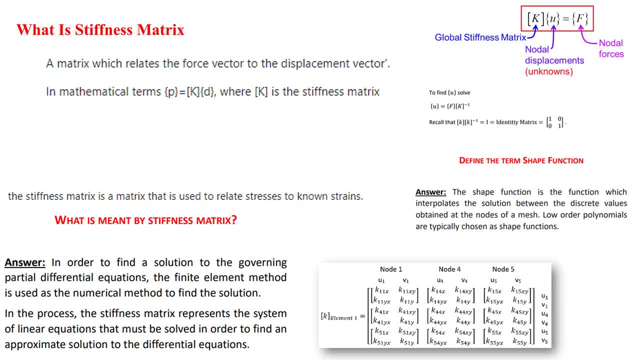 differential equations. the finite element method is used as a numerical method to find the solution. okay, in the process, the stiffness matrix represents the linear equations. okay, so these linear equations will be used to find the approximate results for the differential equations. okay, in short, the stiffness matrix is the formula which will be converted in the form of linear equations to 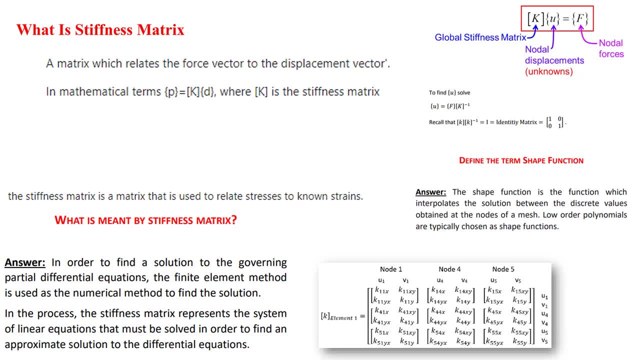 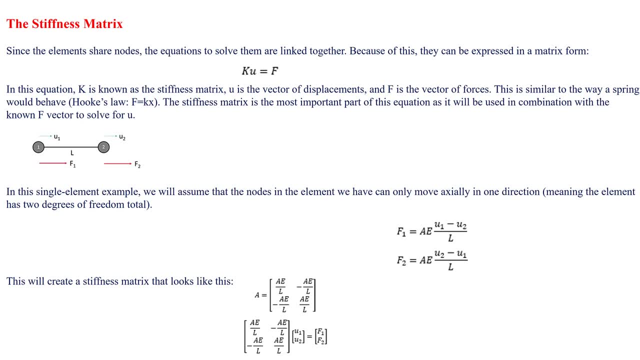 get the results for the differential equations. i hope it's clear, fine. so now again, when it comes to the better explanation of this particular stiffness matrix in depth, we'll consider the same thing. that is okay. element with the two node points: okay, in axial direction. loading condition: 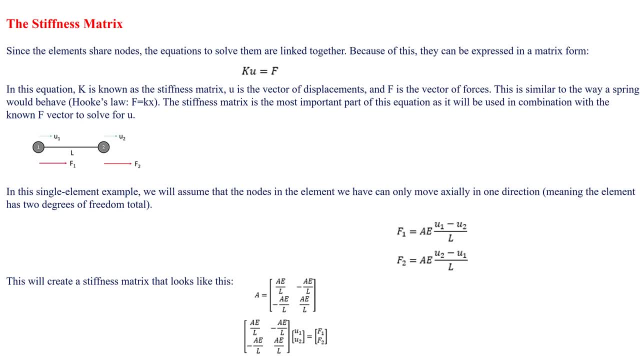 so if i consider the matrix into account, the partial differential equation is: f is equal to k into u, where k is the stiffness matrix, u is the vector displacement, f is the vector of forces. okay, when it comes to a spring, okay, the behavior follows the hook's law. that we already know, that's. 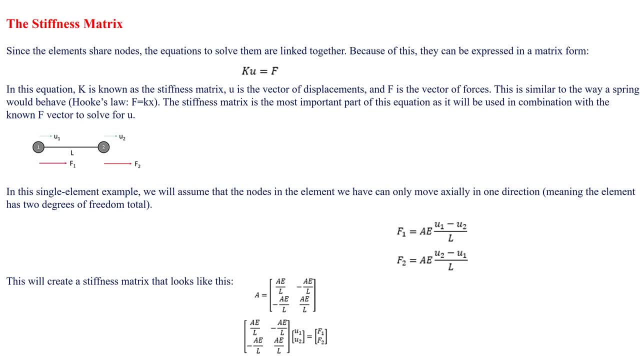 the basics. okay, that is, f is equal to k of x. so same thing. when it comes to the static analysis, the same equation is followed. okay, so we'll consider that a single element, uh example. so assume that, uh, the nodes in the elements have the excel loading condition. okay, so the formula is f1, which is equal to stiffness, matrix is a into. 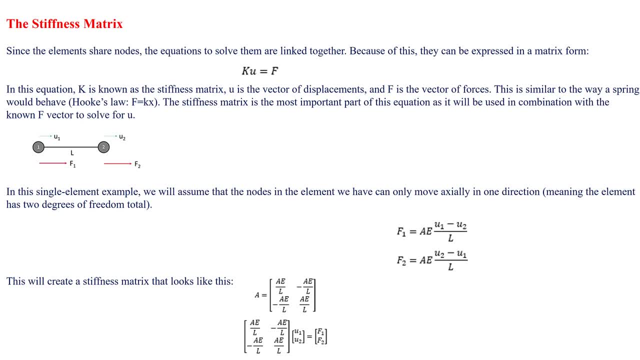 x modulus into u1 minus u2 divided by l. so same thing for f2. okay, when you solve for the stiffness matrix, the formula is here: a by l minus a by l minus a by l and a by l. so once you put this one into the formula above formula, this is what you want to get. 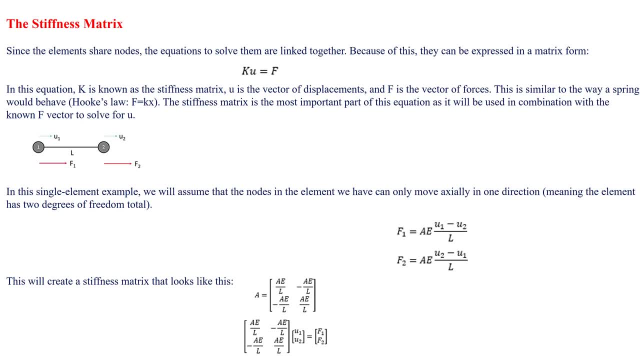 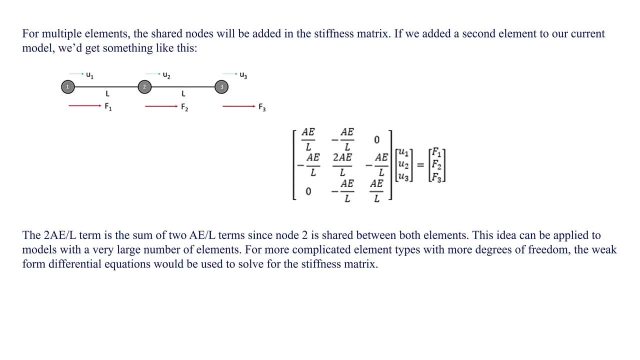 so, in short, the stiffness matrix is the uh simplification of the entire differential equations into the linear equations to provide you the results accordingly. i hope it's clear if you take the same uh particular formula into account, if you solve for nodal forms. so the formula is like this: where 2a by L term is the sum of the a by L term. 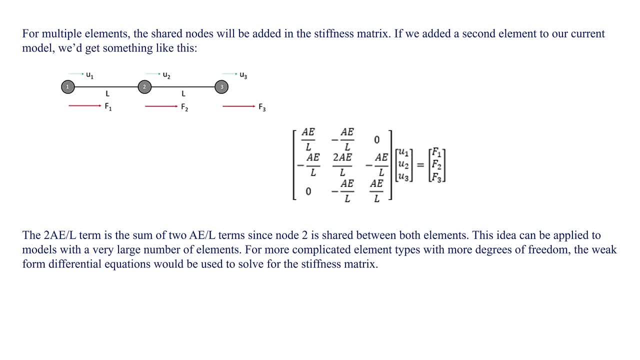 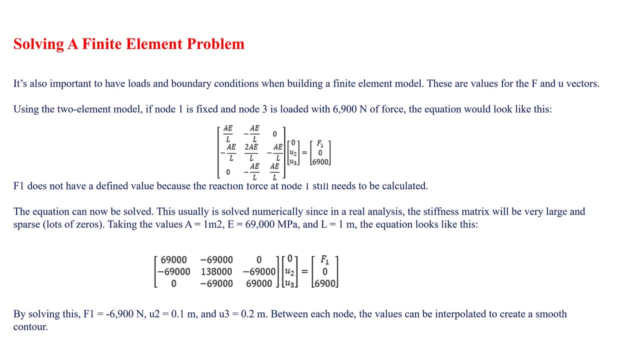 since this particular second node is shared between the both the elements. okay, this will be used for complex analysis as well, so it will keep on increasing. so we'll take the simple example. okay, so here the same condition: two elemental model, so a three elemental model, sorry, so the 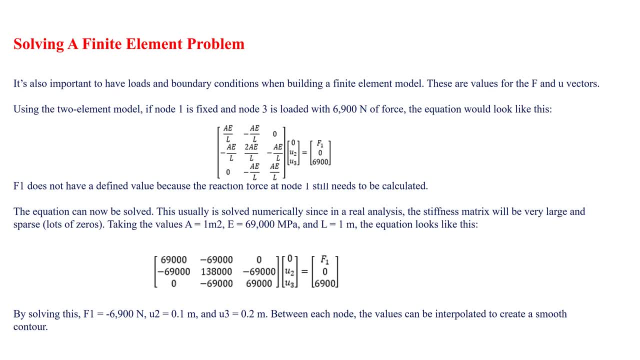 first node is fixed, okay, at the corner. second node is in the middle. third node: we're going to apply the load of 6900 newton force. okay, the equation will be written in the form of this: okay, where f1 does not have a defined value, so that we need to find out right at that location. 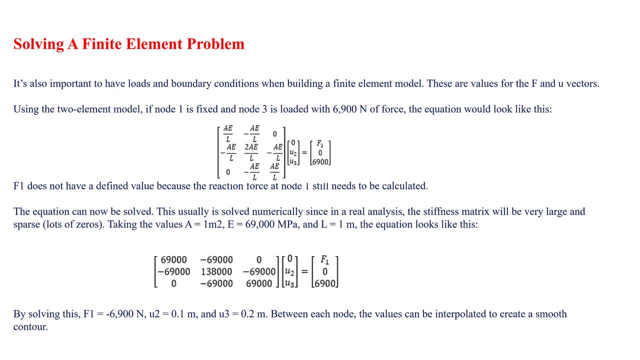 so the equation can be solved by using the following values. like you could see, the area is one meter squared, nx modulus. here is the formula. we already know: 69 000 megapath square. if you just solve for it, you'll get the same thing. so l h is equal to one meter, okay, stress. 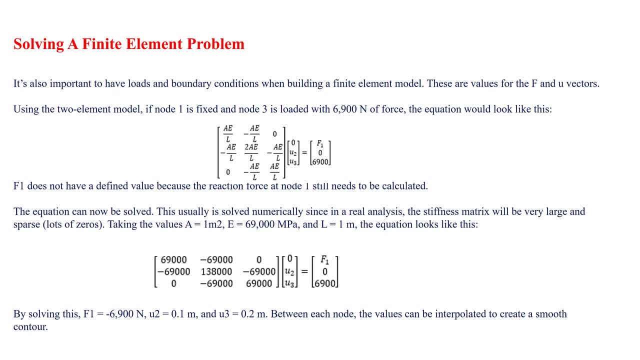 by strain, we can add and we can find out the nx modulus value. it is not that much difficult. so once you add these, all the values inside the formula, you're going to get this formula and if you solve this particular matrix you'll get. f1 is the reaction force at the 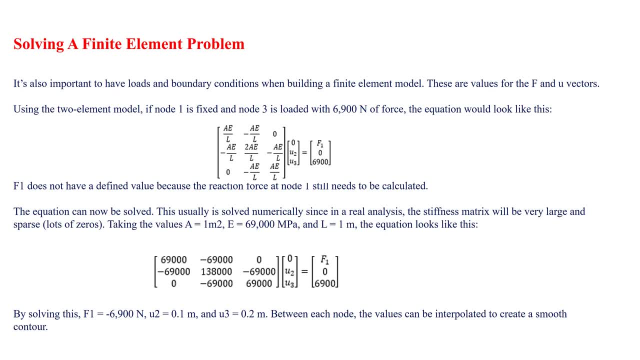 fixed point. it is minus 6900. so basics it is. we already know that we'll get the same value. displacement at the second node, it is 0.1, and displacement at third node, it is 0.2 meter. if you solve the same thing using software, you're going to get the same thing. so if you want to, 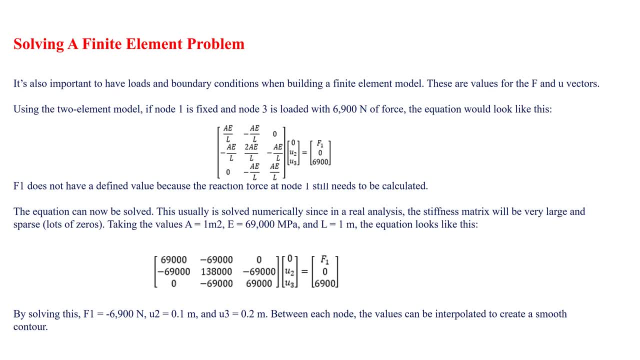 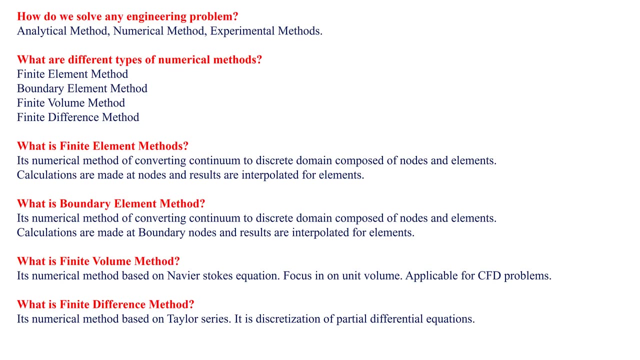 validate it. you can try carry out the same particular problem into the software as well and validate it. i hope you got the clear-cut idea about what exactly the stiffness matrix at the moment. okay, yep, well, so we'll see a few of the questions again here. so how we're going to solve. 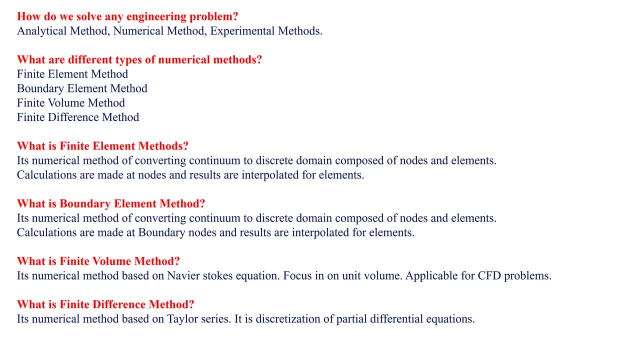 the engineering problems regularly. so there are three methods. one is the analytical method and the numerical method, the software experimental method as well. so these are the three methods. so, when it comes to numerical method, what are the different types? one is the fem, that is, finite element method, boundary element method. second one finite volume method. and 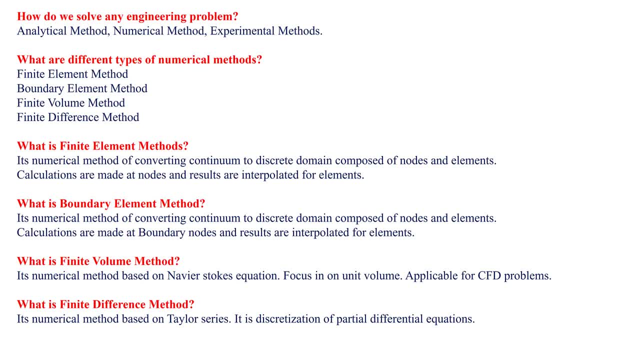 the finite difference method. so, when it comes to the finite element method, what exactly is happening? there is, so this particular entire model will be a consist of the nodes and elements- right, we know that. so the calculations are made for the nodes and the results will be interpolated for the elements. so this is what exactly we're gonna do with fem when it comes to. 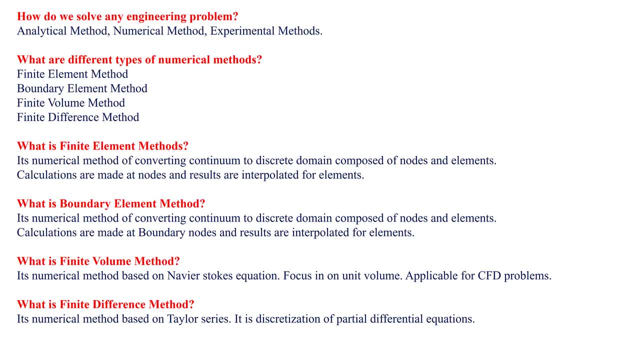 the boundary element method. we're gonna just uh, calculate the boundary node things and we'll just interpret the results with the elements. only boundary nodes will be taken into account here. finite volume method. so this is used to solve the navier stroke equations. okay and applicable for. 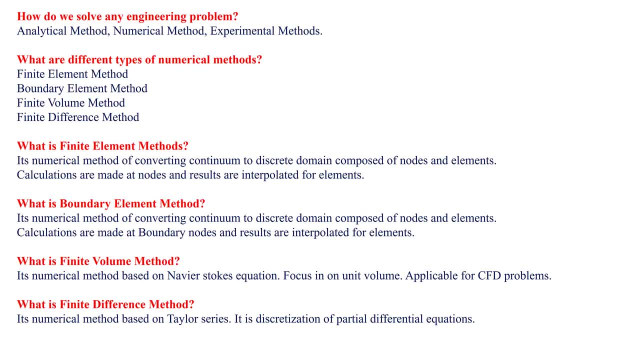 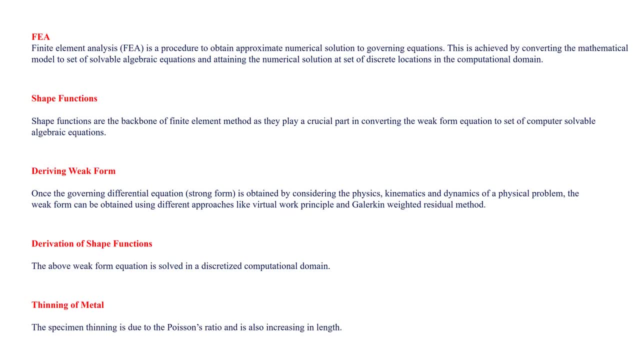 fdm is for the taylor series for advanced dynamic analysis. we use it well. so, as i explained, this fea terms we already know. so what exactly is going to happen? so, when it comes to this shape function, what it is, we need to remember the shape function is going to. 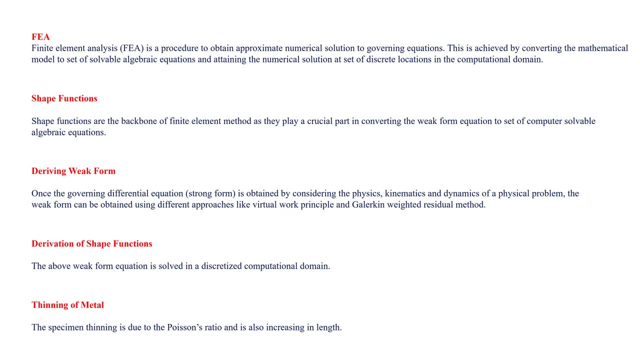 uh take very important role in fea. so what exactly it is? it is the backbone for the finite element method. it plays very crucial role for converting all the uh weak form equations into a set of computers or viable algebraic equations, so that we're going to see later on now how exactly this shape function. 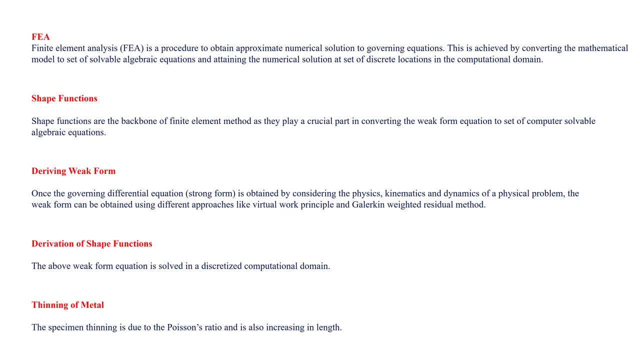 will be formed. okay, first thing is the, the differential equations, which is obtained by considering the physics, kinematics and Dynamics of the app. bring this functions function. we will add one to that thing here. after that it will be termed fb, use bitmapable parameters and in this case the following equations will occur: but we will overwrite our equations, and that hardships because itوي. 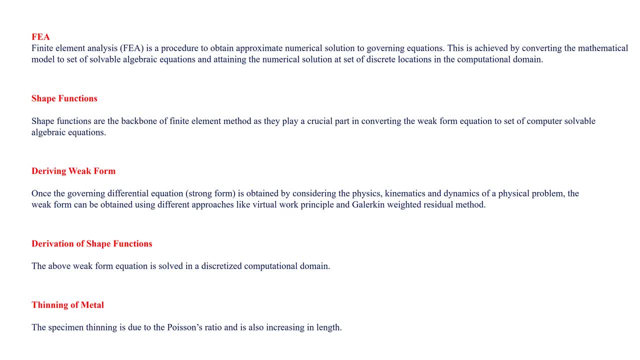 the physical problems. so the weak form can be obtained using the different approaches, like the weak principle or the galilean residual method. okay, these weak forms will be added here and once that is done, we're going to solve it for the shape functions. okay, this all. 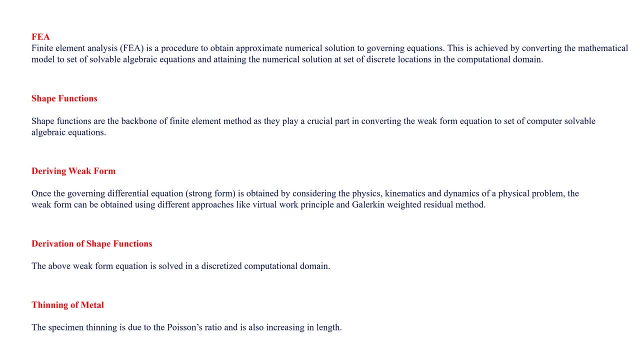 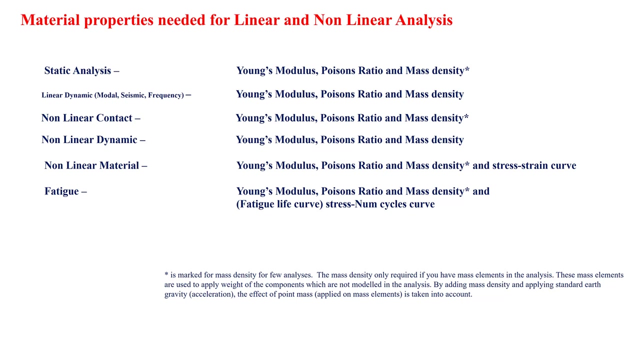 the weak form equations will be solved in a discretized computational domain to get the shape functions. so what is this? thinning of metals? so this particular process where the material thinning will happens and due to the portions ratio, as well as increase in length. okay, very important thing. so what? and all the material properties we need to consider for the linear as. 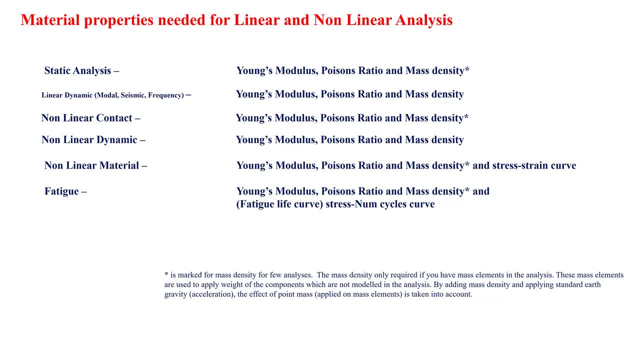 well as non-linear analysis, right, so this is the very important questions, uh, which will be asked during the examinations or any of the interviews as well. okay, we'll see here. the first thing is the static analysis. so, if you consider it only for static analysis, we're going to consider the inks, modulus, okay, the poisons ratio and the mass density. 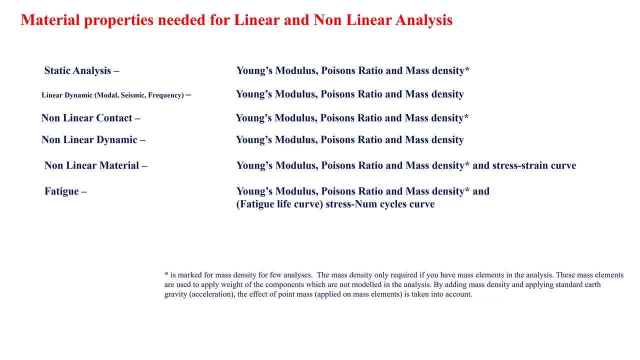 to calculate inks modulus we need the stress by strain value. stress is the yield stress there, yield strength. we can consider and we're going to get the inks modulus right for linear dynamic analysis. what exactly this linear dynamic analysis, which is frequency based? the models is make, okay, the frequency analysis also. so here we're going to. 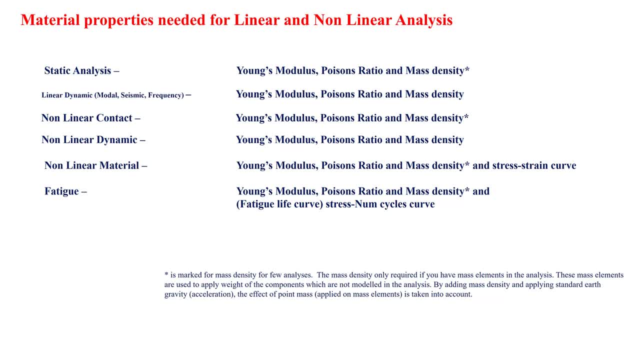 consider the same thing: the x modulus, poisons ratio mass density, non-linear contact analysis. it is also same, okay: poisons ratio, mass density in x modulus. when it comes to non-linear dynamic analysis. same thing, okay. okay, to keep this thing alive, let's look at the next module. 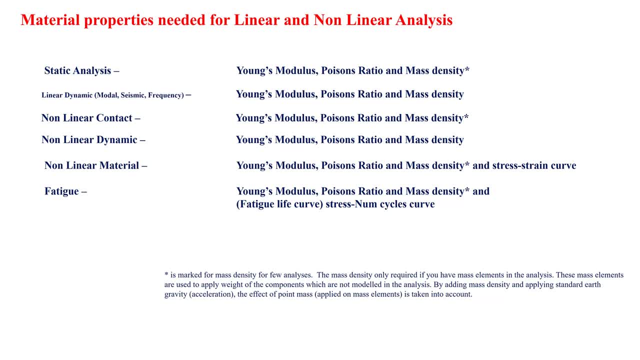 so next lecture is stress strain curve. we're going to see here that the stress strain curve willlist. so for here we're going to see the stress margin curve of stress strain curve. here elements into the analysis like uh, which gonna add the acceleration due to gravity into account. 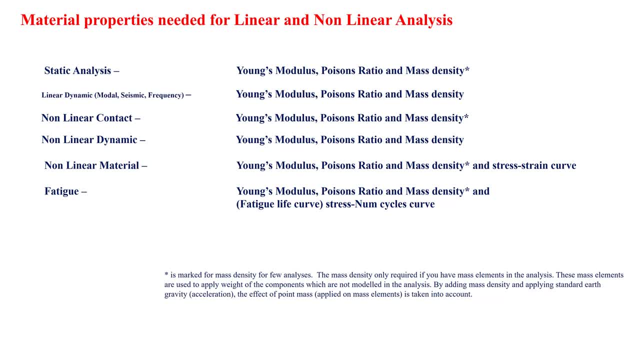 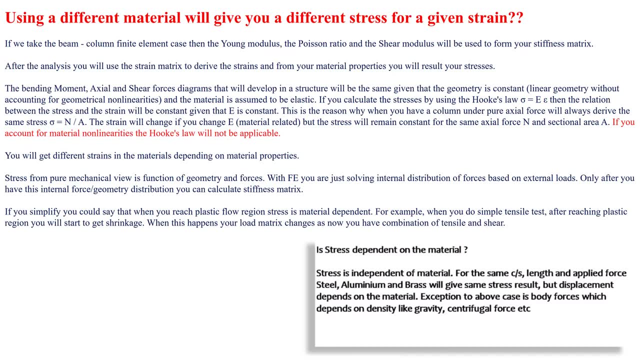 remember that. in short, fine, yeah. so when it comes to this question, so using a different material will give you a different stress or a given strain. in short, the question is: if i use the different material, the stress results will be same or not? so this question has been asked multiple. 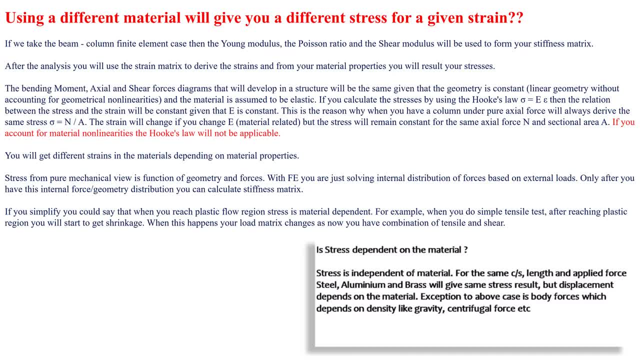 times. even i had gone through this particular question multiple times, okay, so we'll take a simple example here to just explain this. okay, if you consider the beam column finite element case, so the inks modulus, the poisson's ratio and the density will be taken to form the stiffness. 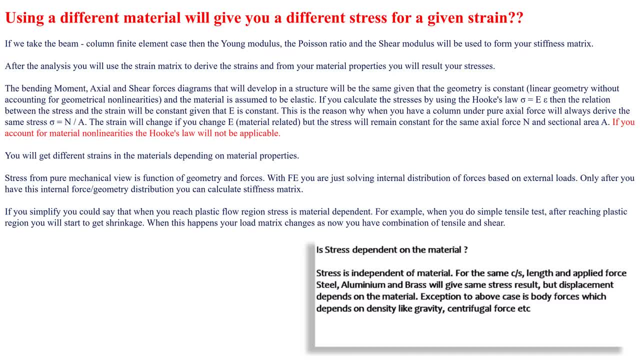 matrix, okay, e by l, you have seen it right. the same thing, the advanced formulas and all so, after you analyze this, so what exactly you do? so you're gonna form the strain matrix to derive the strains, okay, and from your material properties will get the stress distance, okay. 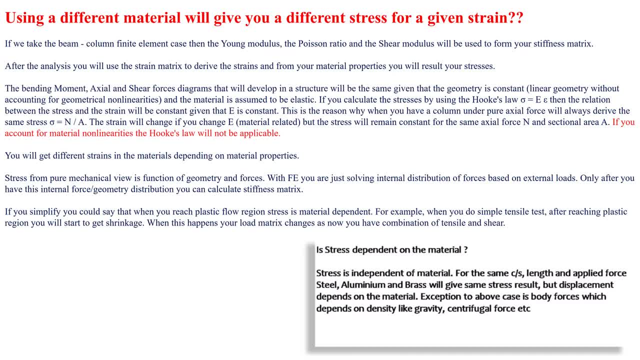 so when you add the bending moment, axial stress uh, shear forces diagrams, so that will be developed in the structure uh, given that the, the geometry is constant, okay. so if you consider this condition, uh, and the material, if you consider that should be under elastic limit, okay, so it will take the 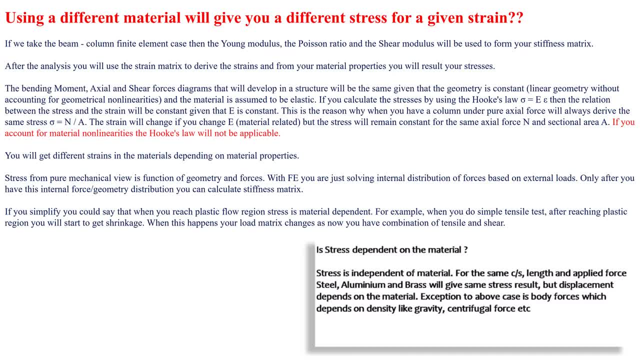 hoax line to account, that is, stress which is equal to x modus into strain. okay, distillation will be taken into account. uh, when? this reason why? when you uh have a column under the excel pure axial loading condition, so the same stress, that is the same stress, will get the same stress, so the strain will change if you change the inks modulus. 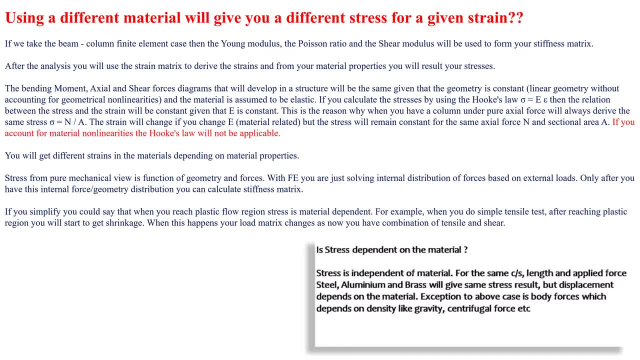 this you need to remember, the strain will remain constant for the same axial force in the cross-sectional area. if you have account of for the non-linearities, the, whatever the hook's line you want to consider, it is not applicable. so under the elastic limit for the static analysis, 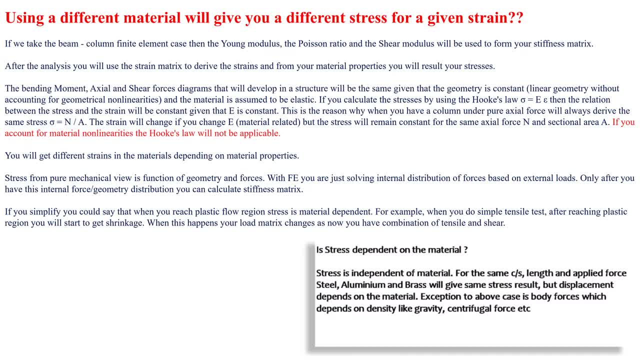 the stress will remain constant in sharp. okay, i hope it's completely clear, so in more convenient way. so if you're going to consider the stress, it is independent of material for static analysis for the same cross-sectional area, length and applied force. so if you consider steel, aluminum, brass, all the materials will get the same stress results but displacement will vary. 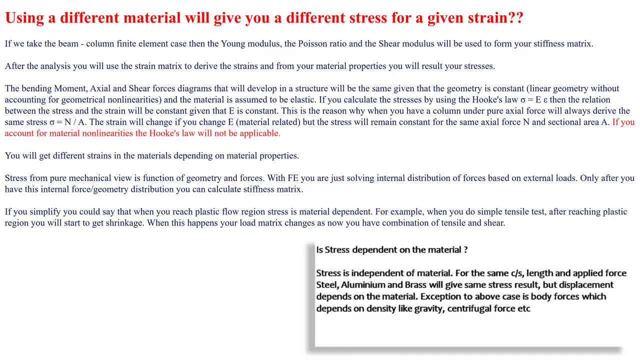 okay, remember that much so if you consider the plastic region. so what exactly happens? there is uh, the combination of uh, stencil and shear force will take place. the metals in case will happen. so this hook's law will not be applicable there, so their stress results will start vary. 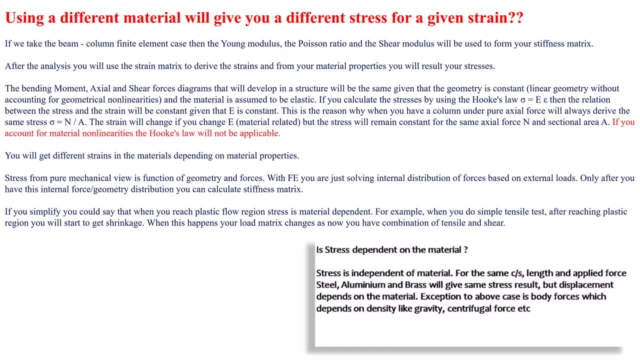 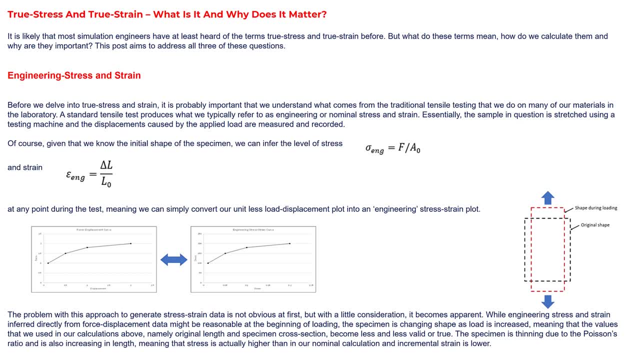 yep, so this is the expression for this question. i hope it's clear. yep, so here the discussions on true stress and true strain and what it does matter, what exactly it is. so this is very important thing, guys. so if you're going to deal with the 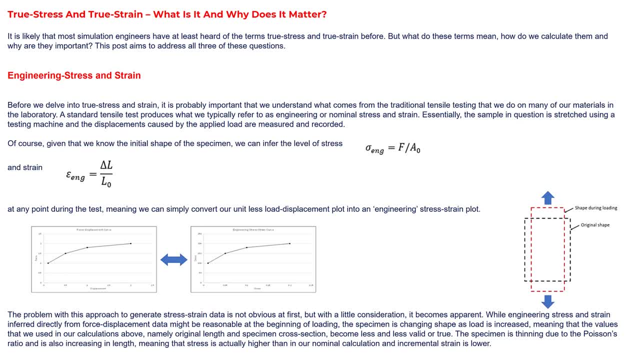 engineering stress strain and the q stress strain. i'll just uh, take you, just uh, like, take you through your past. so if you are the mechanical engineer, you could take your time and you can go on, and and the mechanical engineer or the aeronautical engineer, so you have gone to this universal. 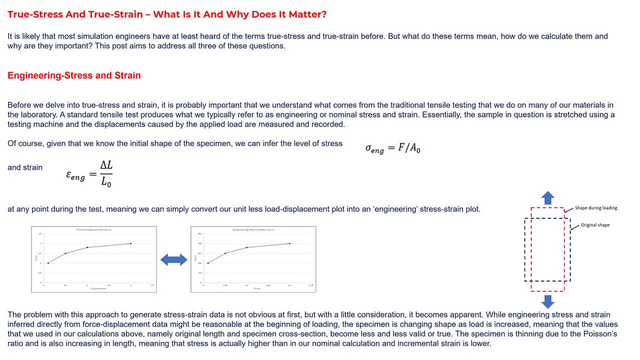 testing machine, right. so where we have conducted this uh pencil testing- so simple, a simple rod- will be taken into account. it will be stretched from one end. one end will be fixed. we'll note on the uh displacement results along with the force which we have planned and we'll convert. 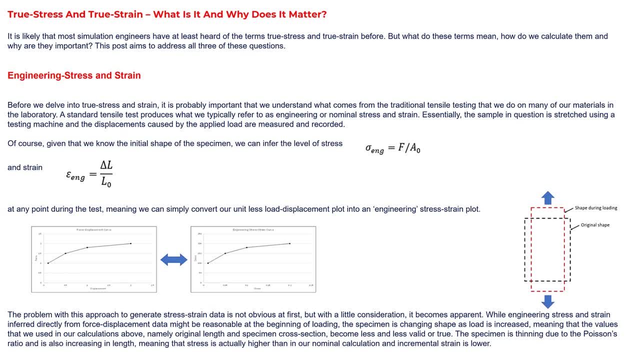 that into the engineering stress and we'll find out the true stress strain values as well by using these things. so that time during that days we didn't know why we are doing so, we simply did like it gets. now, when it comes to c8 domain, which is very important, we'll see exactly how we are. 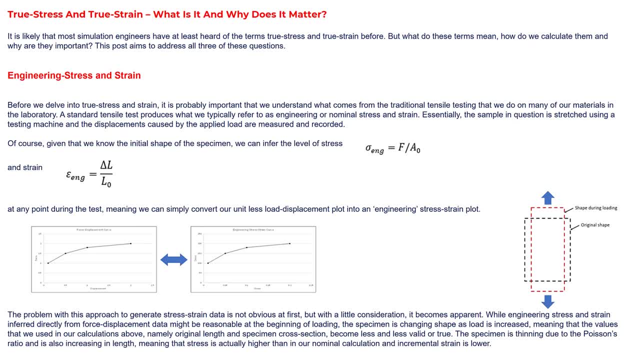 going to implement these things here. okay, so a traditional tensile testing machine. we already know, right, so in the laboratories and all we have used it. so the procedure is to calculate the true stress strain results there. so to calculate this engineering stress and engineering strain, we have used the formula that is, a force divided by area for engineering stress. for 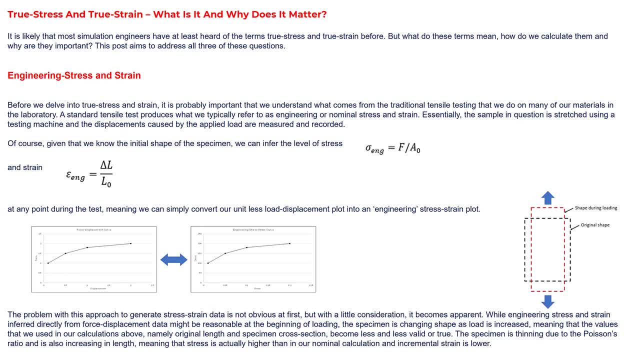 engineering strain. it is changing into the original length. okay, these formulas, okay. so at any point of during this test. so what exactly we have done is we simply converted the load versus displacement engineering stress-strain curve. right, you could see the diagram there. so, whatever the stress strain data we gonna get, it is not obvious at first, right? so 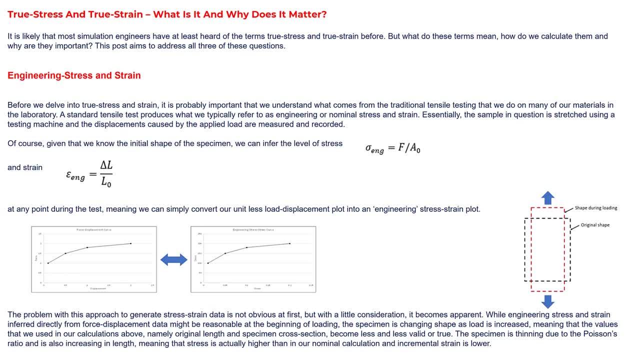 then, with little country considerations, becomes apparent. so while engineering stress and strain so infer directly from force and displacement, data might be reasonable at the beginning of the learning. okay, during the initial stages. the specimen is changing this shape as the load increases. we already see right, so the poissons ratio will takes place there due to the hotel discourse. so 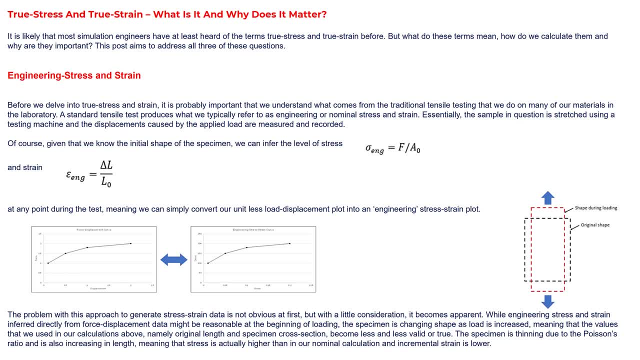 meaning that the values that we have used in our calculation ever, namely original length, we have a fun right for the engineering stress-strain. and when the cross-sectional idea is the original, the cross-sectional area is the original only so this becomes less valid or true. so the specimen is thinning due to the 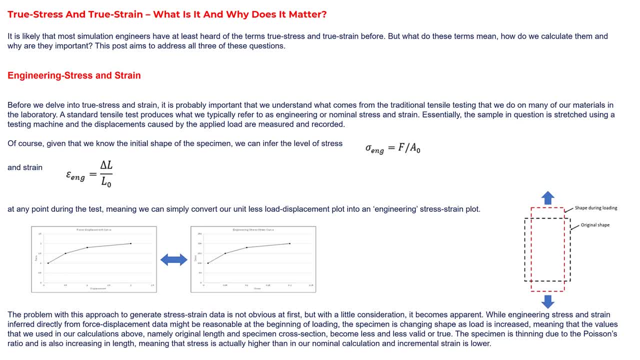 Poisson's ratio, right do. and due to this increase in length as well, okay, meaning that the stress is actually higher in that region and even the, the incremental strain, is lower at that region. so these things we need to consider during this analysis, so to find out this engineering stress strain, now we reach the original. 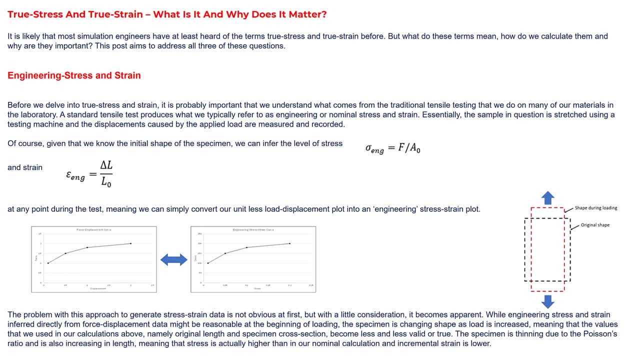 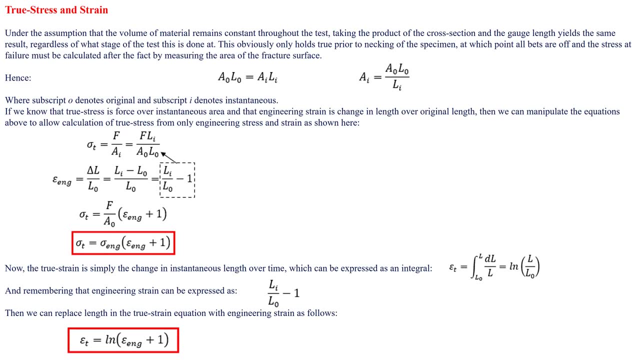 cross-sectional area and the original length for consideration now how exactly we gonna relate this engineering stress strain into the true stress strain. let's see here. you could see, under the assumption that volume of the material remains constant toward the test that we need to consider, if you take that one into account, so the volume is area. 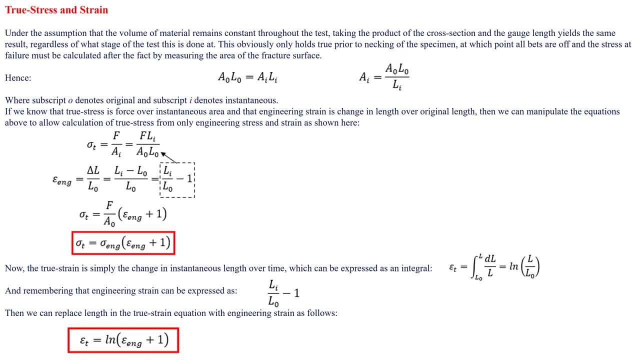 into length: okay. so if I consider the test, after the test, okay, and before the test, this thing: A naught, L naught, and which is equal to EI Li. so when I, if you solve for the area for subscript instantaneous area, the formula will be A naught- L naught divided by Li. just remember this. 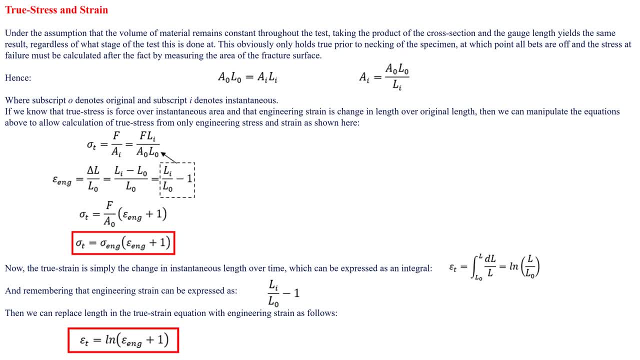 so if you want to find out the true stress strain force over the instantaneous area that the engineering strain is changing length over the original length, we can just manipulate this equation to find out the true stress strain. so to deal with this true strain, which is equal to force for instantaneous 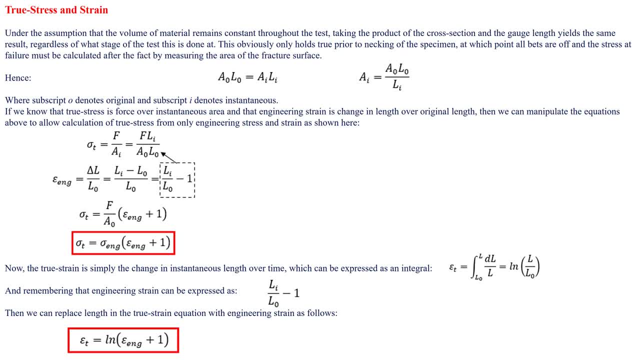 area. okay, when I consider this instance in is area. the formula you can see. just grab it and add it here. Well, for the engineering strain formula is change in length to the original length. It is li minus l0 divided by l0.. So if you just short it off, li divided by l0 minus. 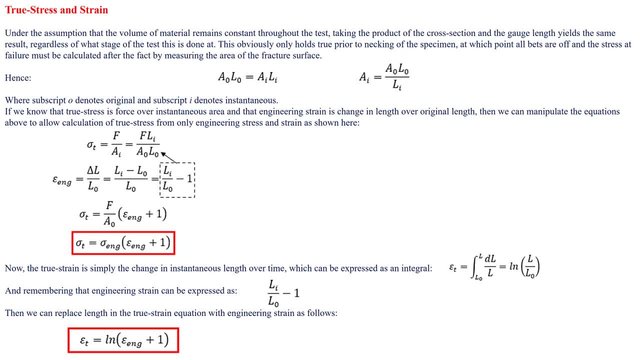 1.. So if you just replace this one that side, engineering strain plus 1, which is equal to the same li minus l0 minus 1, right, So you can write the equation for true stress, which is equal to force per unit area, that is, engineering stress inside bracket. engineering strain plus. 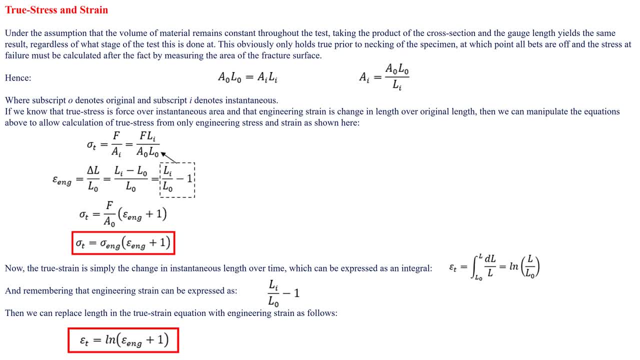 1 for the true stress. quite simple, right. true stress, which is equal to engineering stress plus engineering strain plus 1,- sorry, inside bracket, multiply. So, when it comes to the engineering strain, the formula is ln of l minus l0. and if you solve this, if 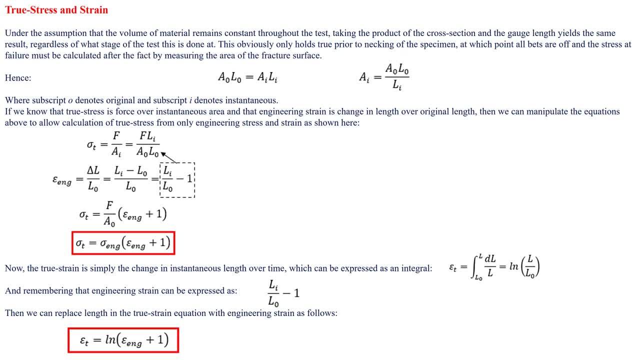 you already know that li minus l0 minus 1 is engineering strain. So you just write the formula strain plus one so you can add the same thing, engineering strain, which is equal to ln of engineering stress plus one. this is how the engineering stress strain and the true strain. 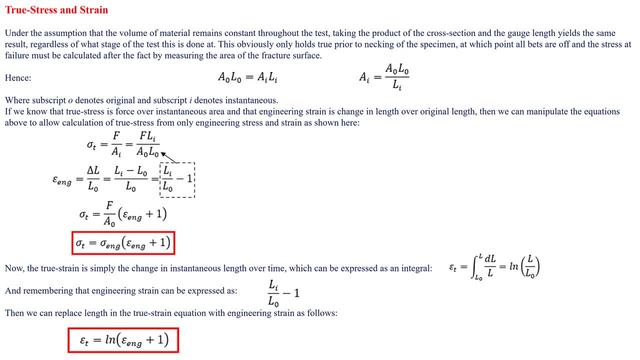 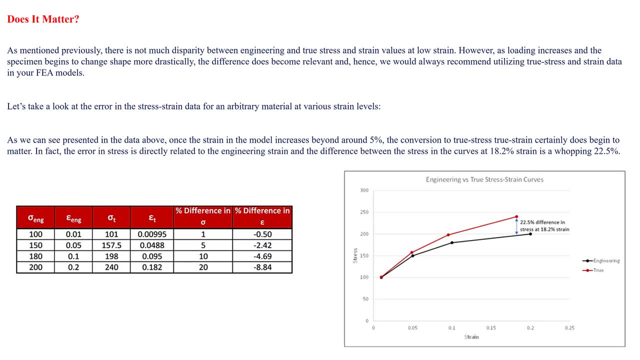 stress strain are linked. okay, so now we'll just deal with the result, so that you can understand how exactly it gonna vary. so does it matter engineering stress and the true stress strain? yes, it does matter. so, as we mentioned before, there is no much difference between the engineering and true stress strain for the lower. 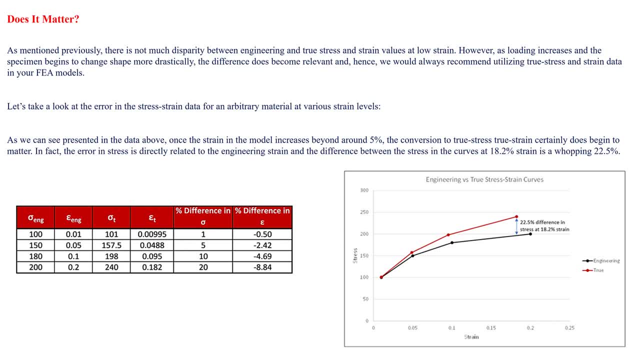 value strains okay. however, loading increases, the specimen begins to change its shape drastically due to Poisson's ratio. this difference becomes relevant and then we need to recommend to utilize the true stress strain data. so if you take the look at the table at the bottom, so when we gonna cross the strain value more, 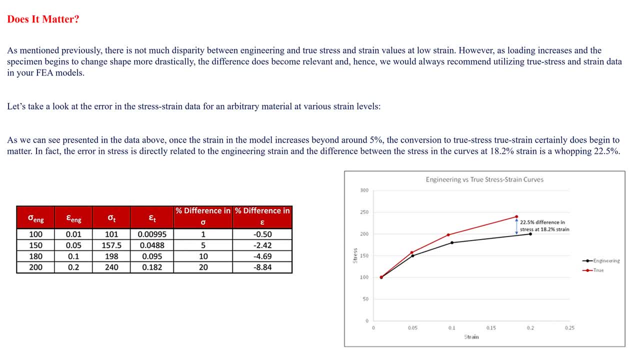 than 5%. you could see the difference. the stress where 18.2%, when it comes to strain, is 22%, so it keeps on increasing. if I consider the 200 engineering stress, the difference is 20%, 22 approximately. right, so true. 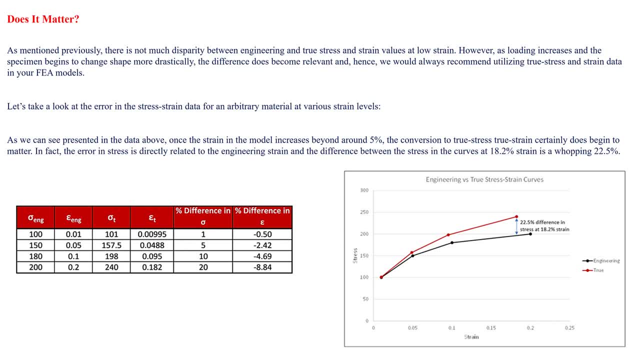 stress is 240 and the strain it is 0.18. right, and when it comes to initial two stages, you could see there is no much difference. 100 and true stress is 1 out 1 and engineering stress is 150 and to stress is 157. the only minor difference is: 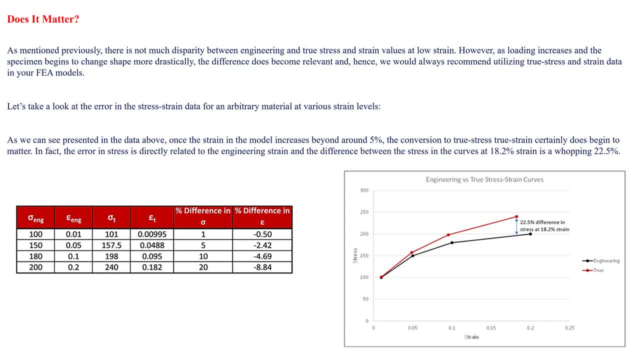 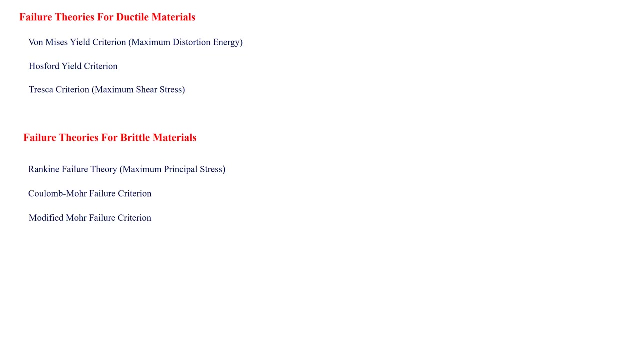 that when it comes to the more, it will completely change. so we recommend, if you're going to deal with the strain over 5% difference, we need to consider the true stress strain curves. I hope it's clear why we might use these things. you have a look. go look at this video, Therese. so for the time we have the 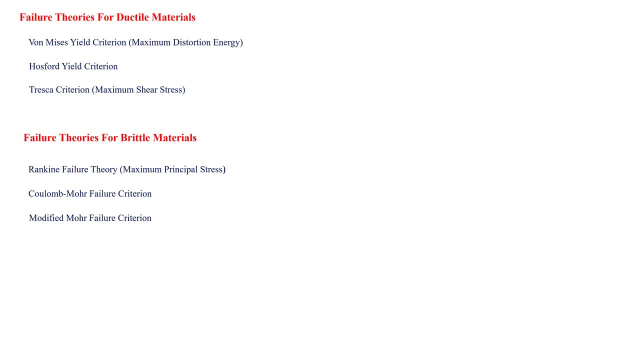 point Moses leave criterion, that is, that is maximum distortion. theory can say Oxford e criterion and prescott criterion. we consider for the ductile okay, most commonly one versus when it comes to the brittle materials rank and theory and the most failure criterion, the column words failure and the 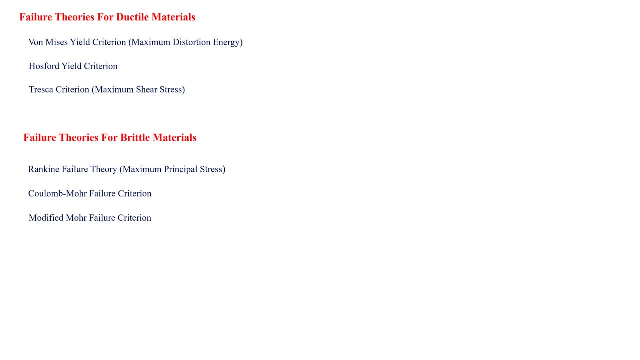 modified force failure criteria we follow. so if you want to know about the, so if you want to know about these things more and more, i have the later on slides, so at the moment it will just go beyond my particular consideration. i'll keep it simple. for ductile we use the one masses more. maximum distortion theory for brittle. 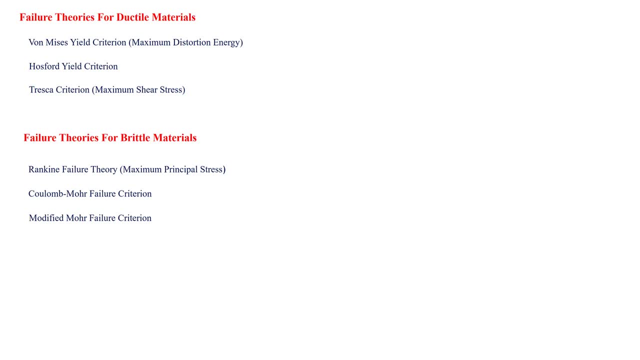 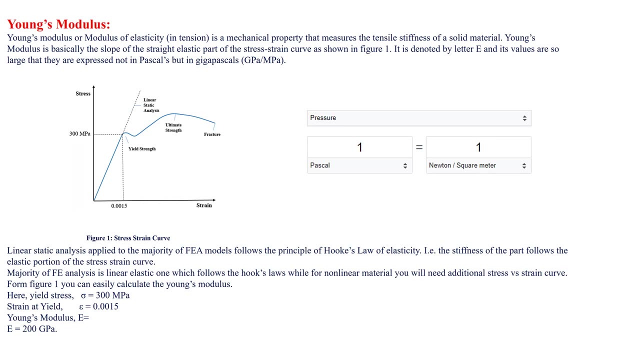 materials, rank and failure and the most failure theories. that's clear. okay, now we'll have a look at the basic terminologies and fea, that is, inks modulus, poisson's ratio and all. so, when it comes to inks modulus, what exactly it is? so, uh, this particular property. 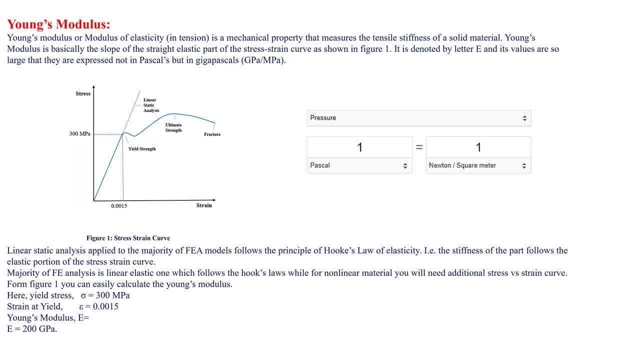 is a measure of tensile stiffness of a solid material. so the stiffness- right, let's go and consider the stiffness matrix. this thing's model is going to be very important role. so basically, it's slope the straight elastic lines to a straight curve. in the figure it is denoted by e. so the in the form of, uh, pascal, we're gonna just measure it one pascal. 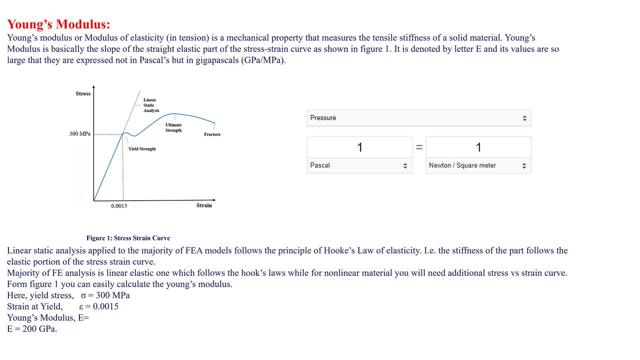 which is equal to one newton per meter square. okay. one mega pascal, which is equal to 10 to 6 unit per meter square, okay. so in the linear static analysis, if you're going to consider that to account, so the fva will follow the hook's law, so it is under the elastic limit. 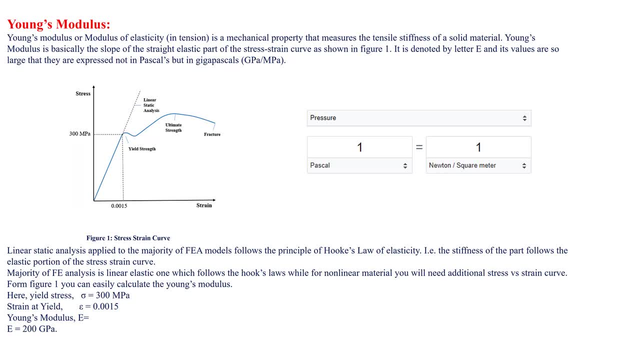 the stiffness of the part follows the elastic portion stress trend curve. so majority of these- all the linear static analysis- will follow the hook's law. we don't need to worry about it when it comes to non-linear analysis. so we're going to consider this stress trend curve along with the hardening rule. okay, now to find out this. inks modulus. 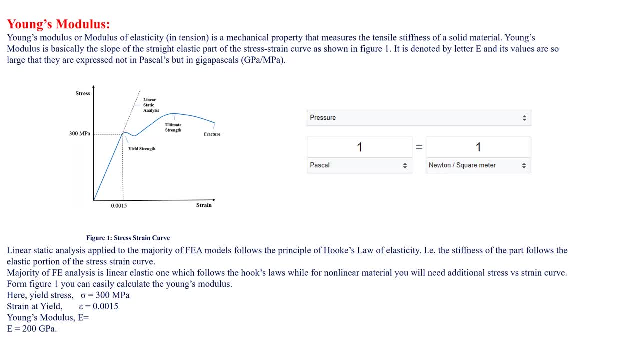 the best formula is to utilize this example, that is, yield stress: 300 mega pascal or steel or whatever you can consider strain, is this value 0.0015. so to calculate x modulus stress by strain according to the hook's law. so 15 into 2 is 30, so you can just add up this one and you will get this value, x modus, which is equal to. 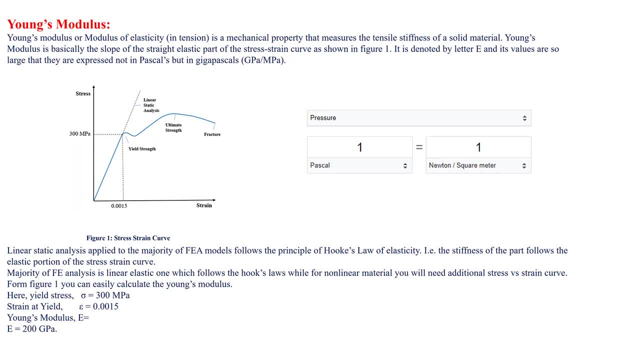 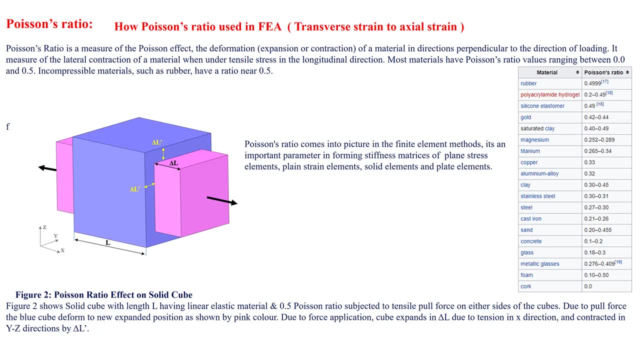 200 gigapascal. okay, this, i can just deal with this. inks modulus. it's quite clear when it comes to poisons ratio. so how does poisons ratio used in fea? the formula is transfer strain to the axial strain, so it is the measure of the poison effect. we can say: 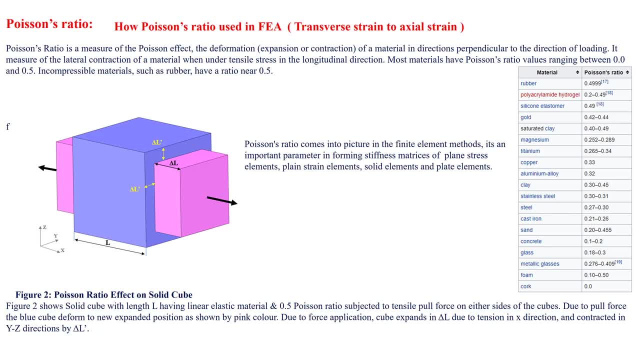 so, in simple, the deformation, expansion or contraction you can consider. okay, so it will be uh, used to measure the lateral contraction of a material when it is under the tensile stresses. okay, in the longitudinal direction. so most of the materials or the metals we can consider has the 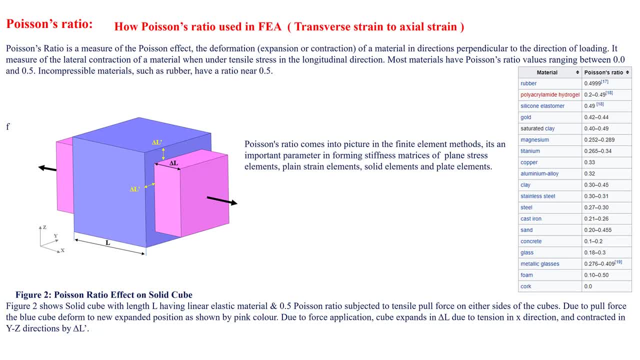 the poisons ratio value from 0 to 0.5. okay, like incompressible metal or the materials we can consider, like rubber, it does 0.5. it is completely uh, incompressible but uh, if you consider this ratio, you can see some of the values there. if you consider. 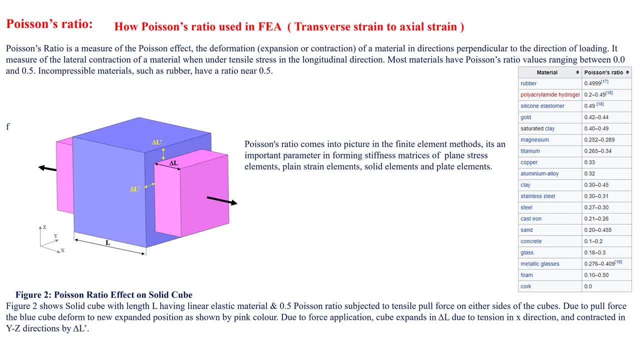 steel it is 0.272.3 and if you consider copper it is 0.33. if you consider the aluminum noise, it is 0.32. if you consider rubber, it is 0.499, it is 0.4. so particularly this poisons ratio will take into picture. 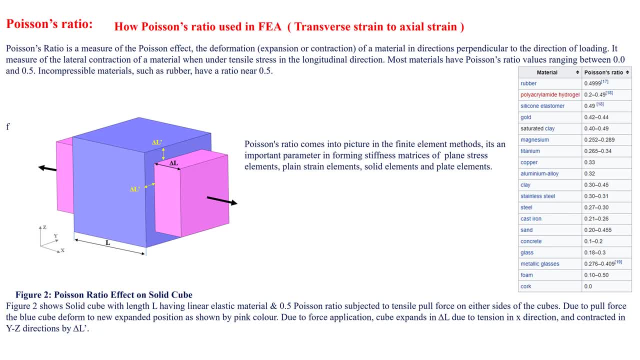 while dealing with the stiffness matrixes of the plane stress, plane strain elements as well as the plate elements. so in the figure you could see right the solid cube with length l, having the elastic material okay and the Poisson's ratio 0.5 subject to a tensile. 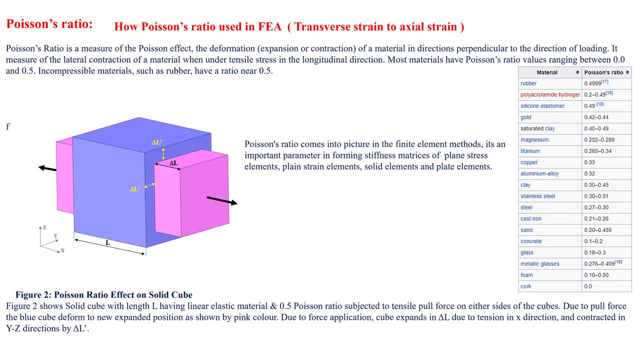 stress when you pull it on either sides. due to the pull force, the blue color cube will deform to form the pink color right where the reduction in the area will take place. due to the force application, the cube expands delta l. due to the tension and x direction contracted in yz direction. 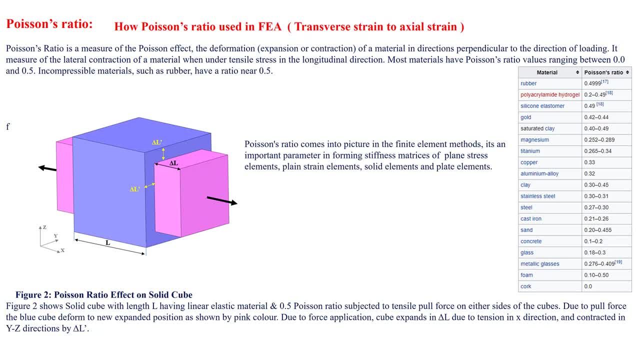 by delta l. I hope it's clear- right: the Poisson's ratio, why we use it and what is the impact. the Poisson's ratio and FE analysis. it is quite simple. so these things we need to know. so, when it comes to basics, I would like to 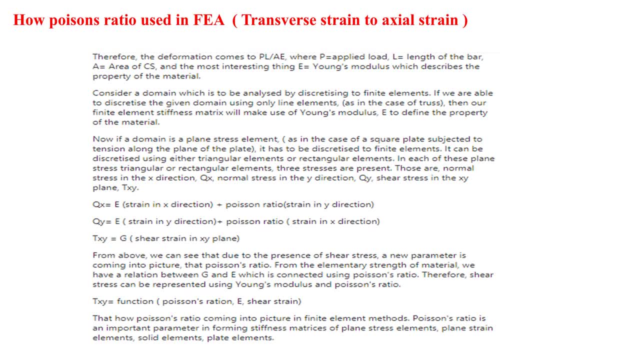 just explain in better manner. okay, so if you consider the same bar example, so it the formula becomes PL by a, where the b is the applied load, l is the length of the bar area of the cross section a. okay, most interesting is thing is the Inks modulus. okay, which describes the property of 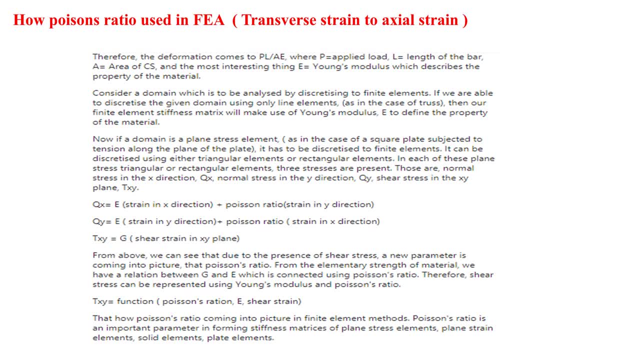 the material. okay, so with respect to properties of material Inks, modulus will be taken into account so we can consider the same domain: finite element analysis. once we discretize this, we will be using the only finite elements here, only line element. we can consider then our element. 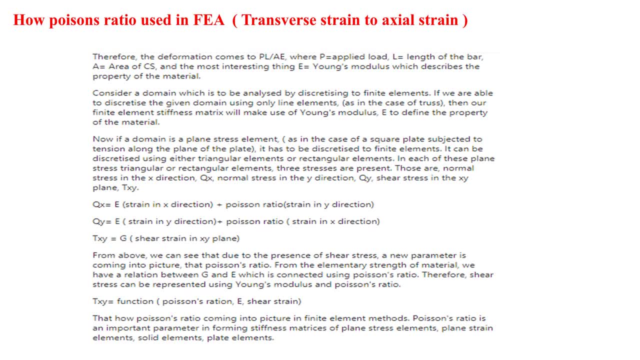 stiffness matrix will make sure that Inks modulus is taken into account for the material. okay, now the same thing. we're gonna consider only the plane stress thickness, like we can consider the 2d elements here to deal with this. tetrahedral or triangular elements we can consider to deal with this. so 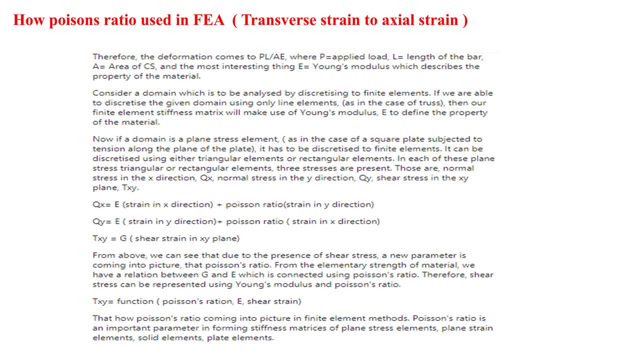 once we deal with this, we can have the original in the form of stress along X direction, stress along Y direction, normal direction and shear stress along X? Y plane. so if we consider these things, the formula will be: it will be taken a token like a strain in X direction for 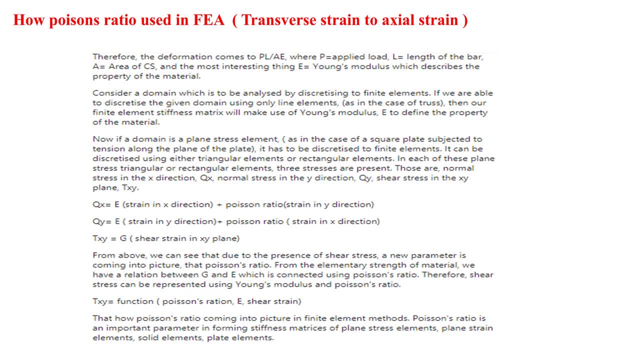 stress along X and the Higgs modulus plus Poisson's ratio into strain in Y direction. same thing for stress along Y direction and the shear stress value, pure stress in X- Y plane and the Higgs modulus. okay, so once you're going to consider these things, or the shear stress can be represented using the. 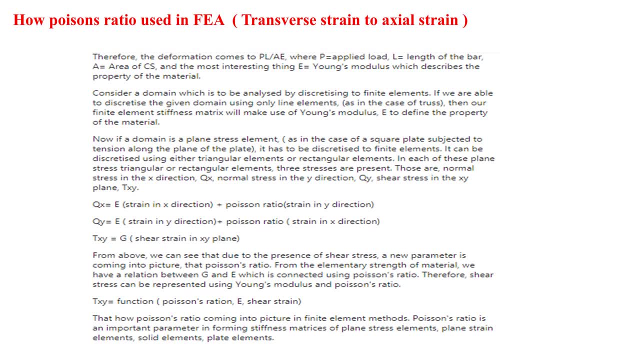 Higgs modulus, as well as Poisson's ratio. so, when you consider these things into account, the Poisson's ratio coming to picture okay. so, which is very important while considering these, forming the stiffness matrices for the plane stress, plane strain and the solid elements, as well as the plate elements. 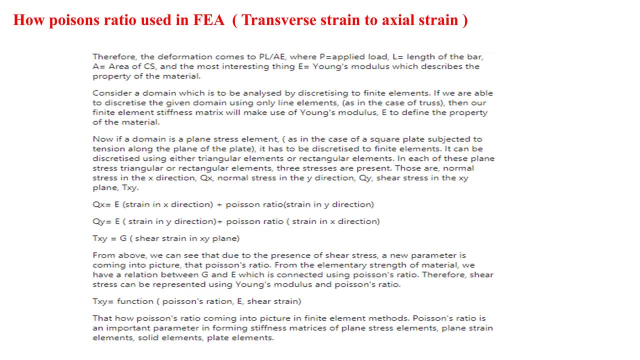 okay, hope it's very clear so why we consider this Poisson's ratio into account while dealing with the FE analysis. okay, so this plane stress, plane strain, normal stress, normal strain and the shear stress are going to come into picture to solve these things, to form the stiffness matrix, and all this poisson's ratio plays very important role. 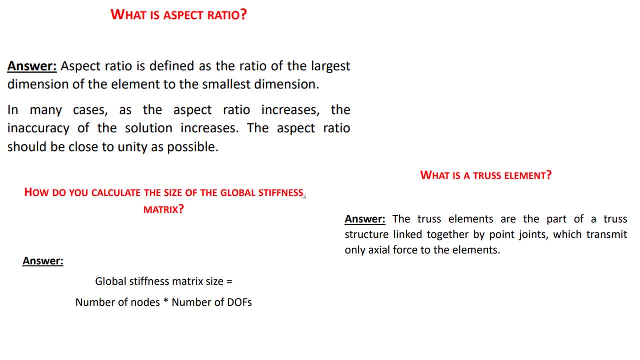 okay, we'll see this aspect ratio, what exactly it is once you consider the aspect ratio to account. so it is the ratio of the largest dimension of the element to the smallest dimension. if i consider the triangle, or the bottom length is largest, one right to the perpendicular length. so this ratio should be equals to one or unity. so 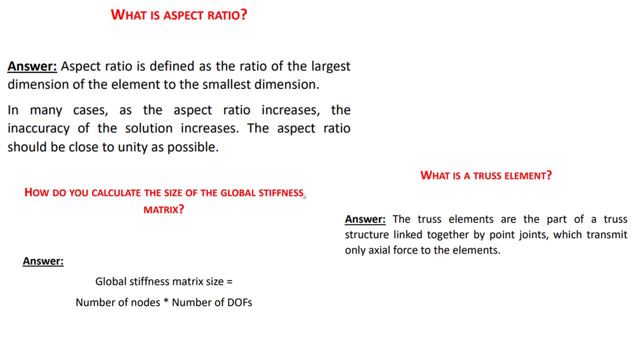 more it is distorted from one, the lesser the result. accuracy, remember that, okay. what are the truss elements? so, uh, these are the uh part of these structures linked together by joints so we can consider the one day elements so, which transmit only the axial force to the elements. 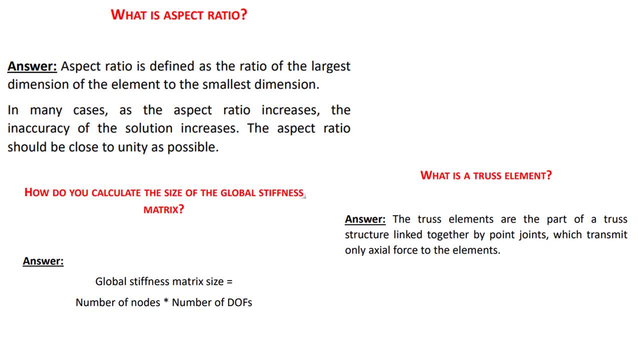 not all the forces. so this stiffness matrix, the formula is already, you have seen, that is it when i take the number of nodes into account and the number of degrees of freedom, and it will solve the entire stiffness matrix to give the results the former strain, or the displacement, or the stress. fine, so very. 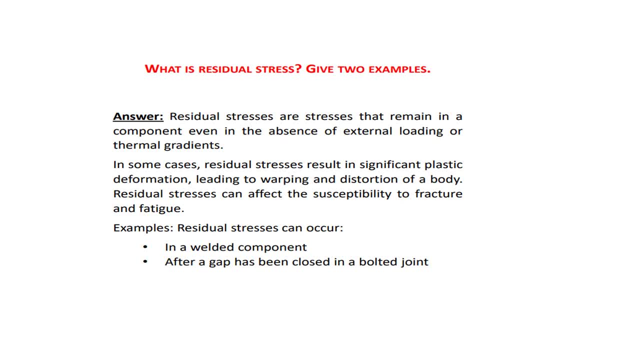 important term is one more, that is, residual stress. so what it is? so this exactly, is the stress which will remain in a component even in the absence of the external loading condition. thermal gradient, we can say: okay. in some cases, threshold stress results in the significant plastic deformation, okay, leading to the wall page or the distortion body. 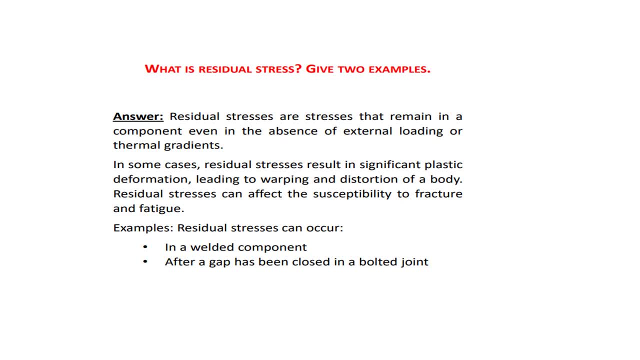 so, again, it might even affect for the fatigue as well as the fracture consideration. example in a weld component: okay, where you're gonna have this residual stress even after gap has been created, uh, due to this particular boarded joints. so they're also gonna form this residual stresses. 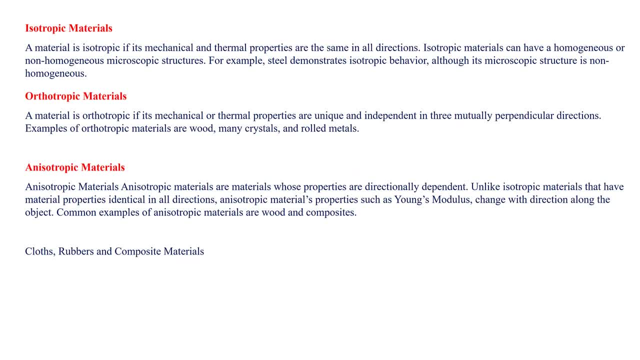 okay, finally we'll see about this. uh, types of materials, we're gonna consider, that is, isotropic materials, orthotropic and anisotropic materials. so when it comes to isotropic, the material properties, the thermal properties as well- mechanical and thermal are the same in all the directions. remember that very important thing. so simply, we can consider steel and other.